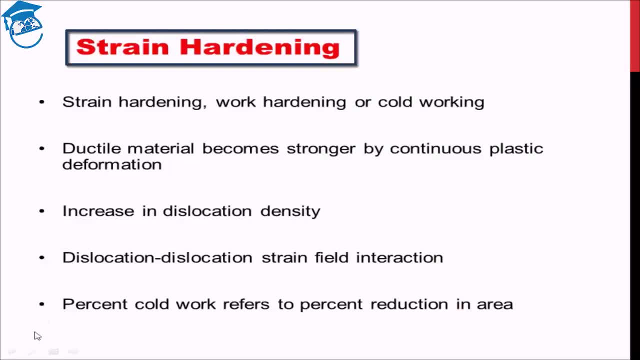 focus will be on what is known as strain hardening. Now, strain hardening, we will discuss what exactly it is, but to begin with, strain hardening is alternatively known as work hardening or cold working. Basically, the name suggests that it is a hardening process. right, and this is hardened. 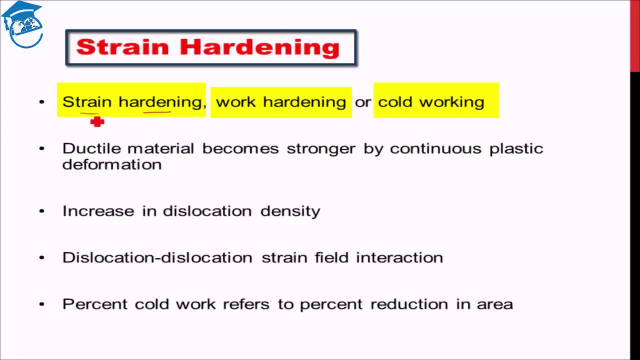 due to internal strain being generated. Alternatively, this name means work. hardening means you work on the material, that is, you impart energy into the material. as a result, the material hardens. Cold working. the name is a bit different from the other two. This means that the working 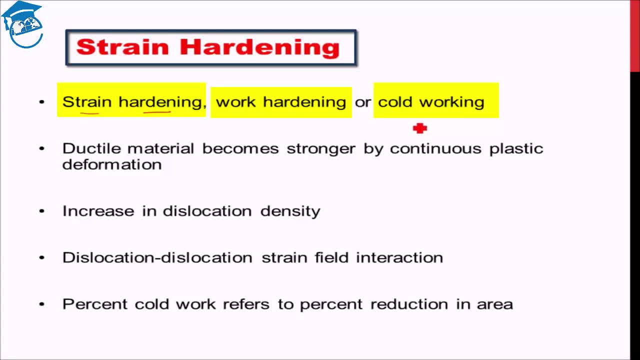 process takes 4 days of 3 days. the deformation of the material gets carried out. So the deformation is carried out at a relatively low temperature. You cannot go at elevated temperature for strain hardening to occur. Now the idea is that ductile materials- if you strain harden it, then the ductile materials 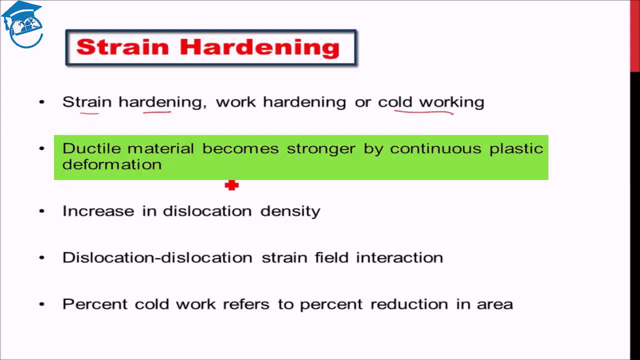 will become stronger due to continuous work. Now the idea is that if you strain harden the material, the structure of the structure becomes final. You cannot go ahead and strain it. So the structure of the structure becomes final. You cannot go ahead and strain, harden it. 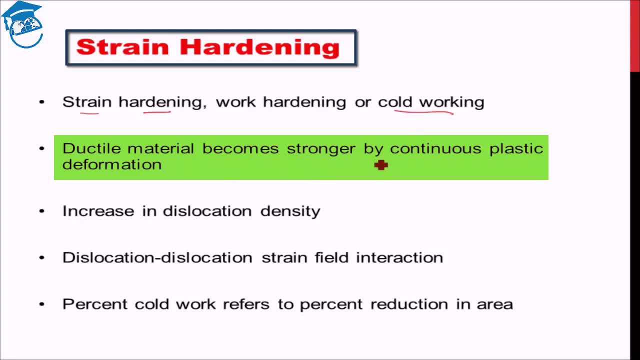 plastic deformation. So the idea is: continuous plastic deformation leads to strengthening of the body. Okay, we understand that continuous plastic deformation leads to strengthening, but why should it lead to strengthening? What exactly is happening when you are continuously deforming the material? When you start to deform a material before starting to deform the material, the 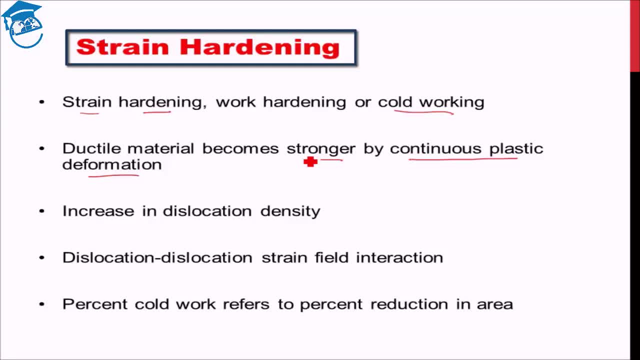 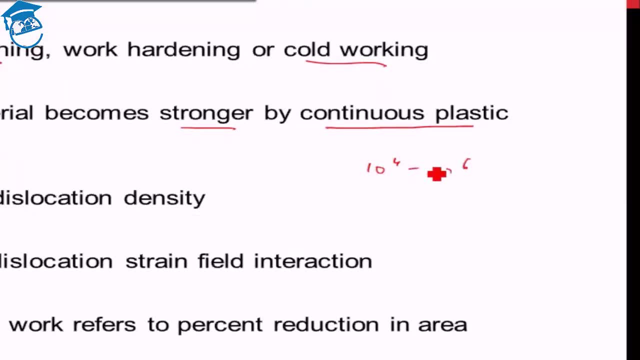 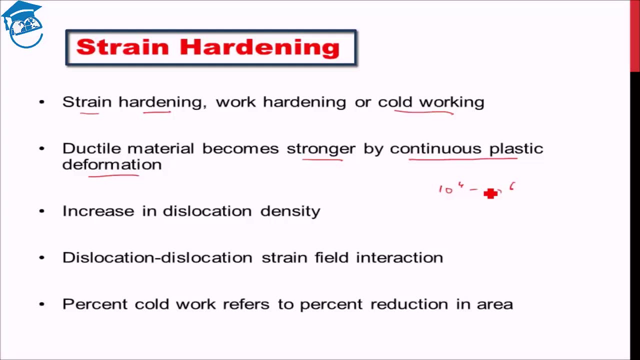 material has a specific number of dislocations. okay, In the order of 10 to power 4 to 10 to power six dislocation density range. but when you start to work hard in the material, you are plastically deforming the material as a result. what? 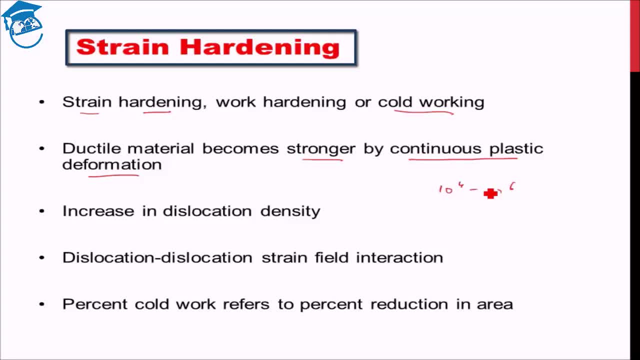 is happening. the number of dislocations starts to build within the material. Plastic deformation leads to generation of new dislocations- effective number of dislocations within the material. then you have a specific number of dislocations. the material is increasing. Now this increase in dislocation density, the dislocation density 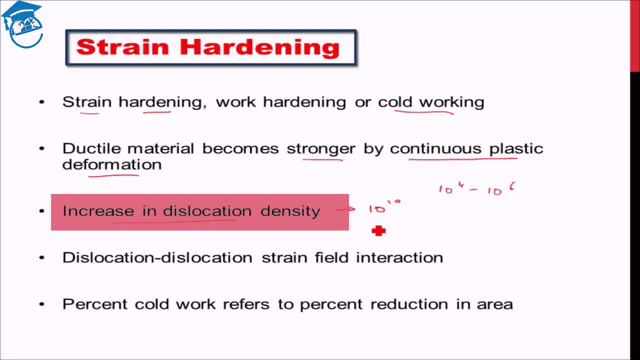 reaches around 10 to the power 10 when sufficient work hardening is done. Now this increase in dislocation density leads to dislocation-dislocation interaction. Even in the initial stage, when dislocation density was like this- 10 to the power 4 to 10 to the power 6, there were dislocation-dislocation. 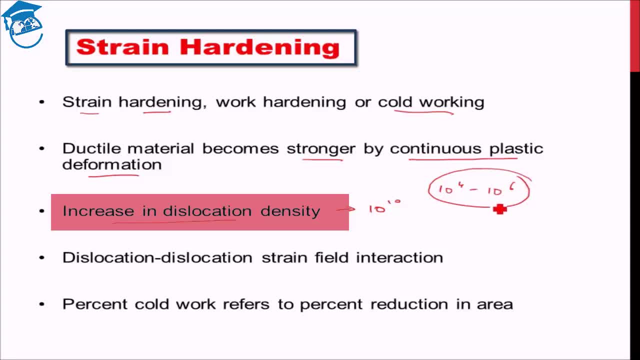 interaction and there was strengthening due to that. But now, since the dislocation density has further increased, the amount of dislocation-dislocation interaction will be much more than initially, and more the number of dislocation-dislocation interaction, more will it be difficult for the 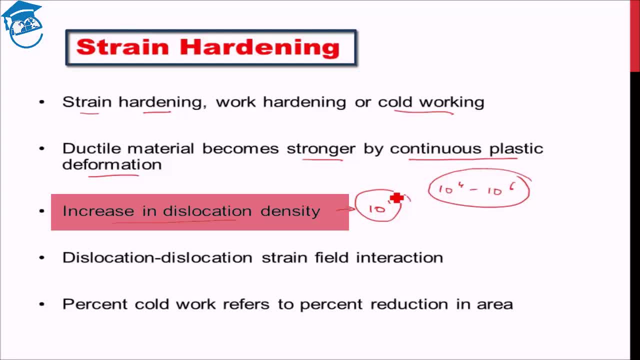 dislocations to travel through the material. More will be the pinning down of dislocation, more will be the energy requirement and the Y и Ukraine, Lee Ku hungry. other people in India also asked the same question: Where exactly does the cyclic distribution of Bol Glm occasionally start and start getting здrapiece, and ¿ Which way do we changec theев analysis? 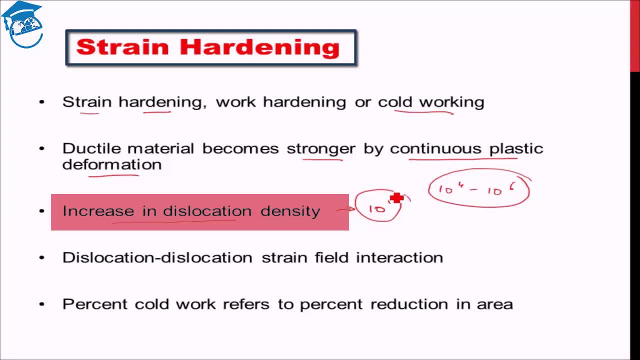 stress requirement for the dislocation to move and further plastic deformation to happen. So see what exactly is happening: You start to deform a material, Dislocation, density starts to increase and that starts to try to prevent further deformation of the material. So the deformation of the material kind of restricts further deformation from happening. 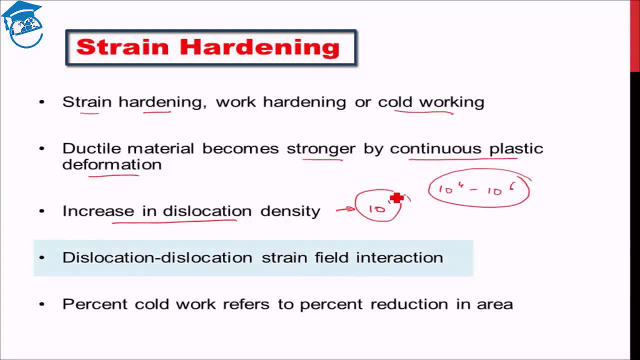 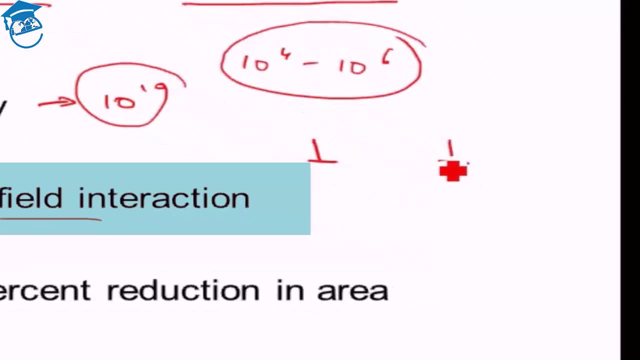 by increasing the dislocation density and leading to dislocation-dislocation strain field interaction. This we have already discussed. The idea was that two dislocations of the same sign will repel each other right. Two dislocations of same sign will repel each other and two dislocations of opposite sign. 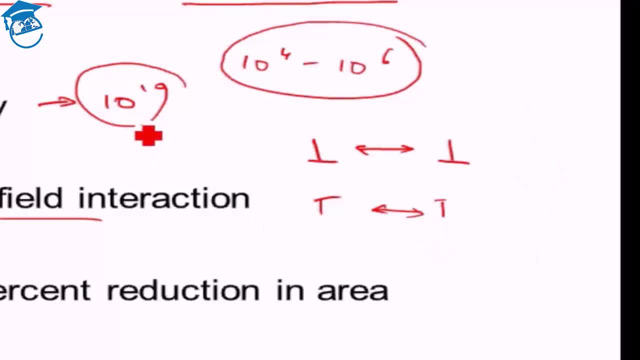 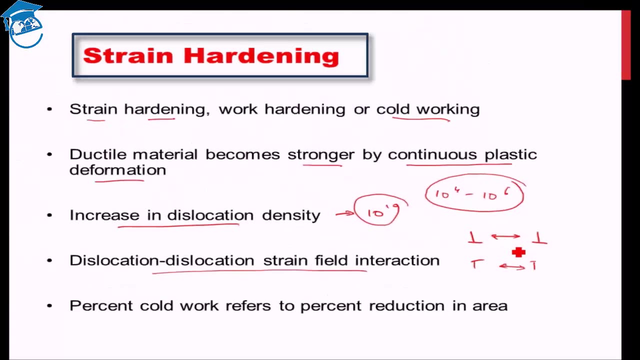 will actually attract and cancel, But since the dislocation density is much, much higher, there is a lot of chances that opposite dislocations will interact right. So this is the basic idea, or basic physics behind strain hardening. Now, the amount of strain hardening that you put into a material is defined by the percent. 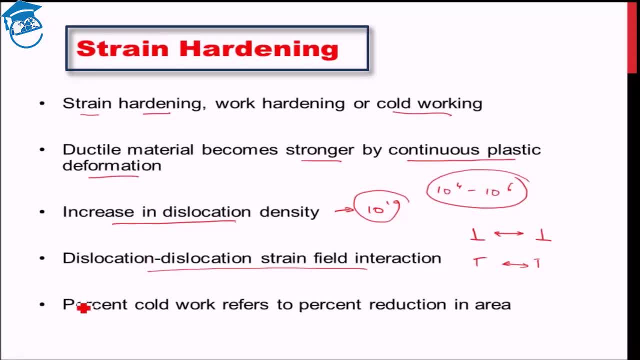 of cold work you do on the material. Now, what does percentage of cold work mean? Percentage of cold work refers to the percentage of reduction, Okay, Or percentage of reduction in thickness of a material Strain hardening. there can be different ways to deform. 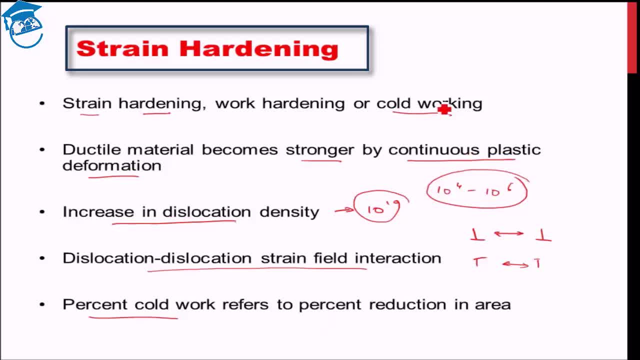 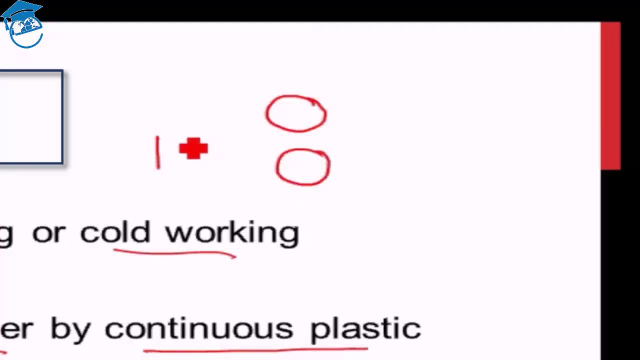 One of the standard way is to cold roll the material. So, cold rolling what you do? basically you have rolls through which you pass the material right. So this thickness, let's say, is T1.. But this distance is less than T1.. 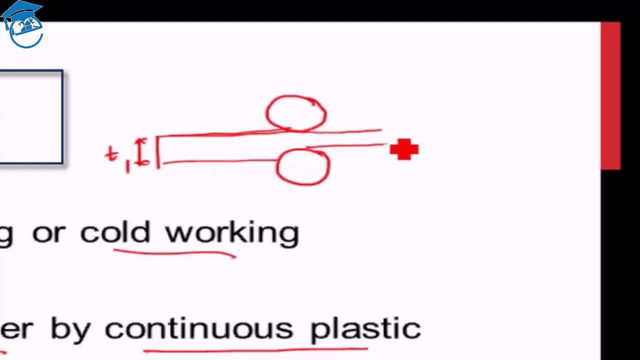 Therefore it kind of thins down on passing through the rolls, So this becomes T2. Where T2 is less than T1. And by continuously passing the material through smaller and smaller roll, more and more work hardening is being done. And this reduction in area, rather the reduction in thickness, means that the thickness of 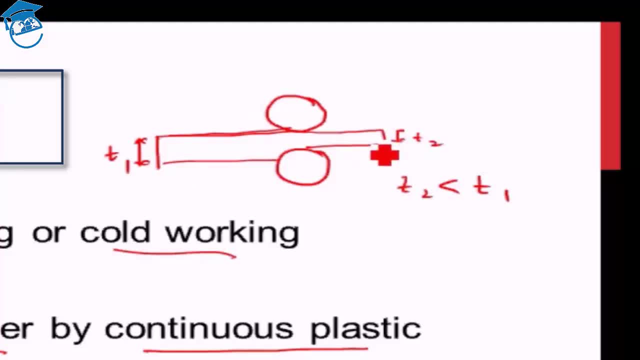 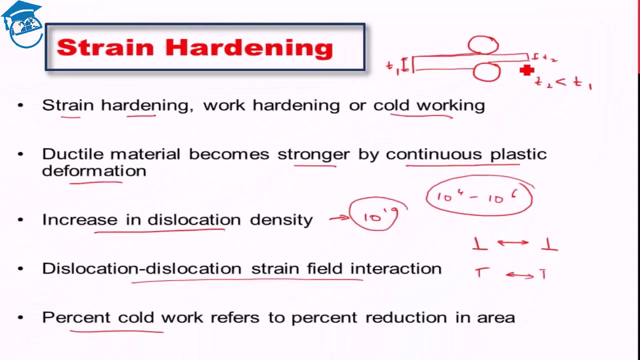 the material is less than T1.. Okay, It manifests itself as an increase in area in the other direction, because volume needs to be constant And that is kind of the percentage of cold work that you are doing on the material. Okay, Now that we have the fundamentals of strain hardening, let us see what is the influence. 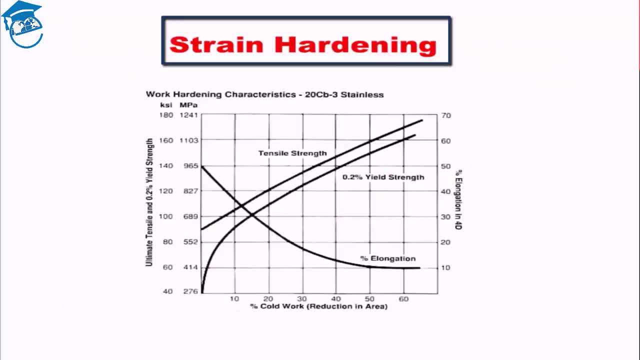 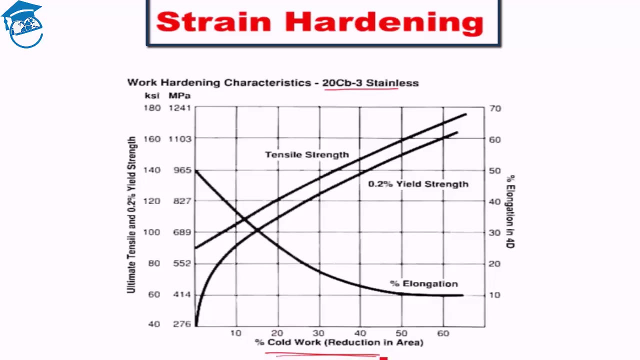 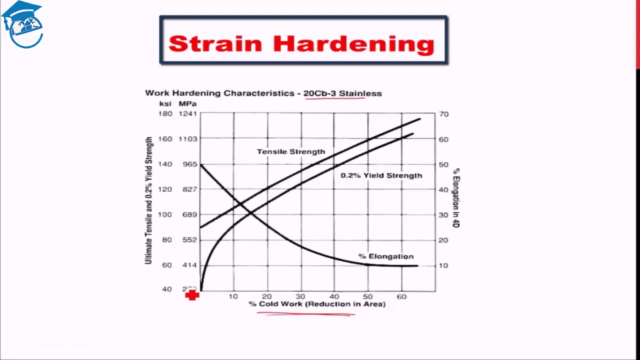 of strain hardening a material. This is an example which I have taken up. This is 23 stainless steel. Okay, And here what we see? this axis, the x-axis, is percentage, cold work or reduction in area. So here we have done reduction in area, plotted against three things. 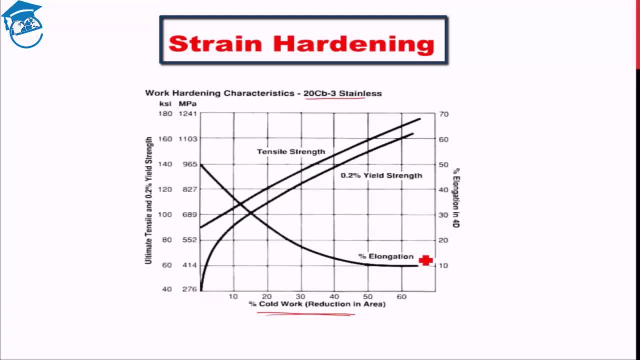 One is: what is the ductility measurement or percentage elongation? What is the yield strength And what is the tensile strength? Previous slide one thing I forgot to mention: that, due to strain hardening, the strength increases, Right Strength increases, but the ductility decreases. ductility decreases. 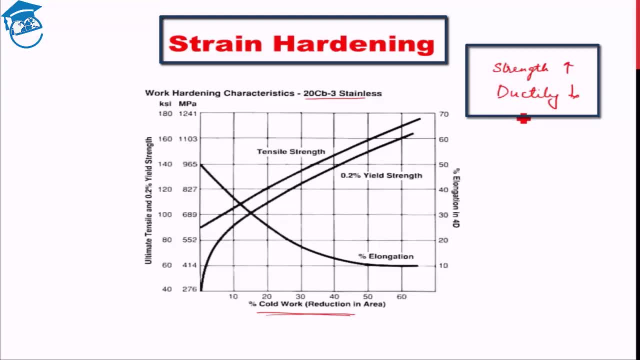 So this is the compromise you have to do. while strain hardening, You lose ductility. That is seen here As the percentage cold work is increasing. the ductility, or percentage elongation, is continuously decreasing, from about 50% and 0% cold work. 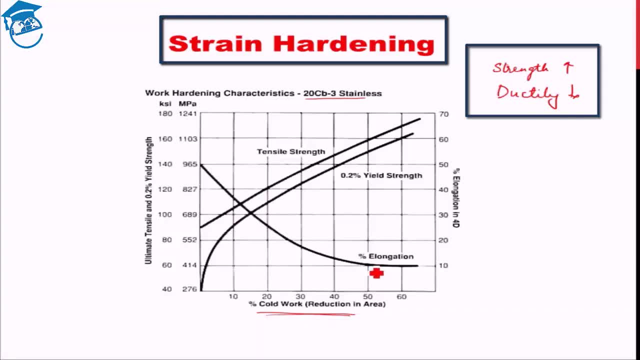 to about 10% or 50% cold work. On the other hand, both the strength- the 0.2% yield strength and the ultimate tensile strength- both seem to increase continuously as the percentage of cold work is increasing. So 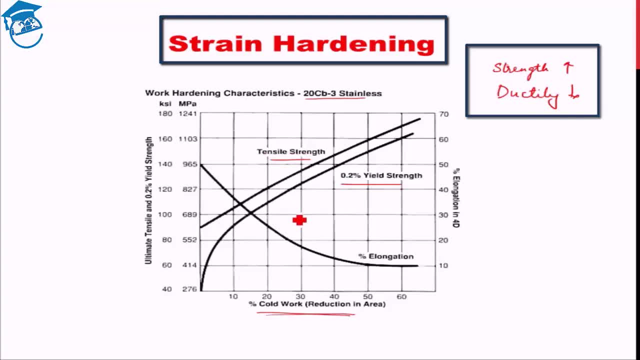 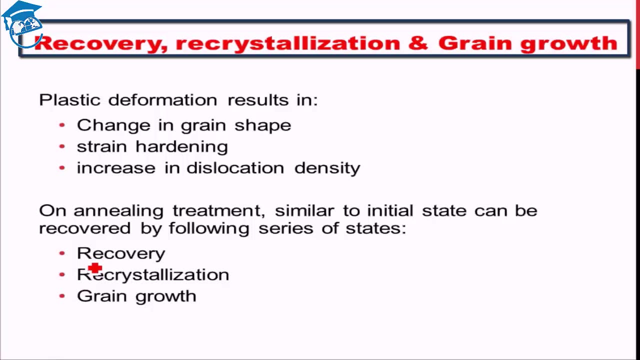 this gives you a clear idea about the effect of strain hardening on the different characteristic of the material. Now let us discuss something which is known as recovery, recrystallization and grain growth. What we have seen till now is that the strain hardening is taking place that is leading to. 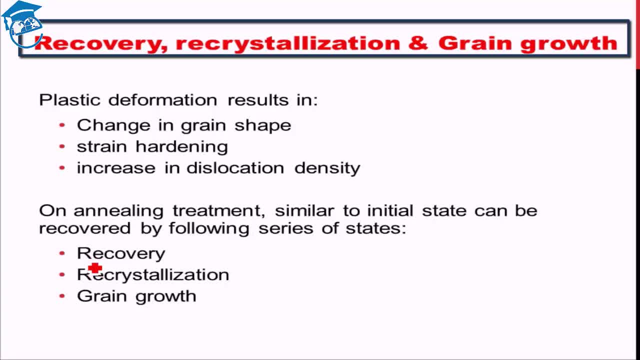 increase in strength, but it is compromising with the ductility of the material. So by continuous strain hardening you are actually reducing the ductility of the material to maybe unusable range. The ductility becomes so less that you cannot use it to any practical. 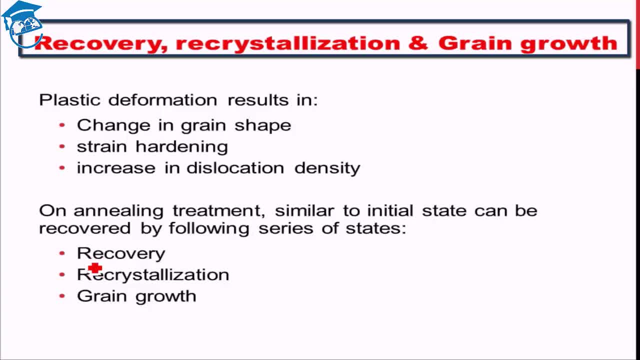 application. So there has to be some method by which you can kind of improve the ductility by compromising on the yield strength a little bit, but the effective result is that the yield strength is not compromised by that much as the improvement of ductility takes place. 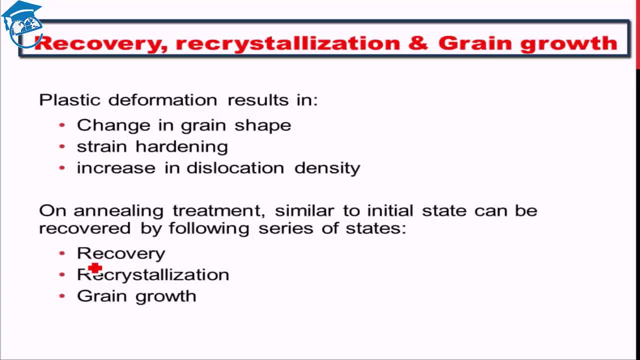 That is done by the process of recovery. Recovery and recrystallization. What happens during plastic deformation? Let us see what exactly is happening during plastic deformation. When you plastically deform a material, several kind of changes are taking place in the material. 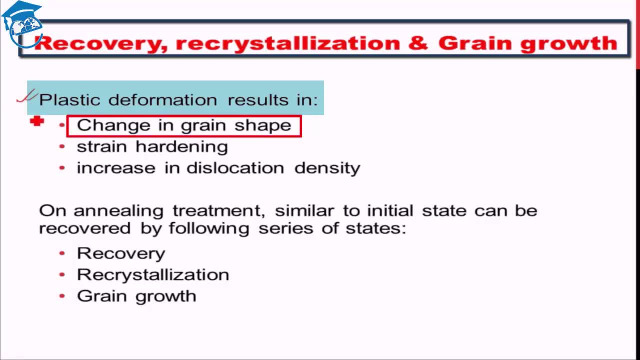 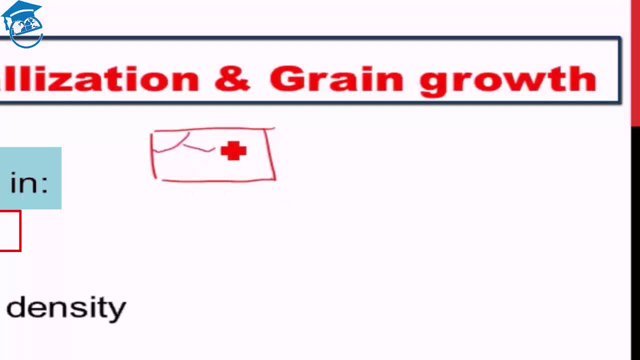 First is there is a change in shape of the grains. So normally speaking, grains are equiaxed, So they are more or less circular kind of shaped- circular shaped. Now, if you pass this through, roll, if you strain, harden this material, what will happen is that it will elongate right and the equiaxed shape now becomes elongated grains. 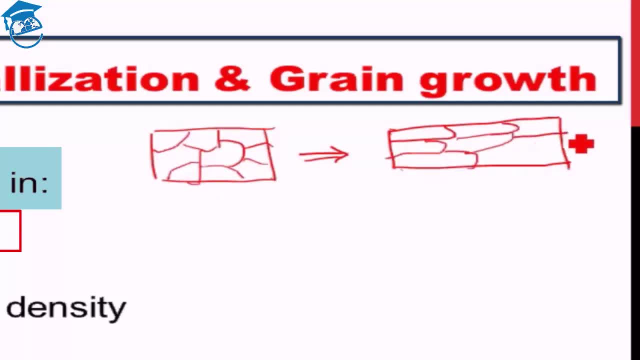 You no longer have equiaxed grain. The elongation takes place in the direction of the rolling. So if the rolling was done in this direction, the grains becomes elongated in this direction. So basically, plastic deformation leads to change in the grain shape. 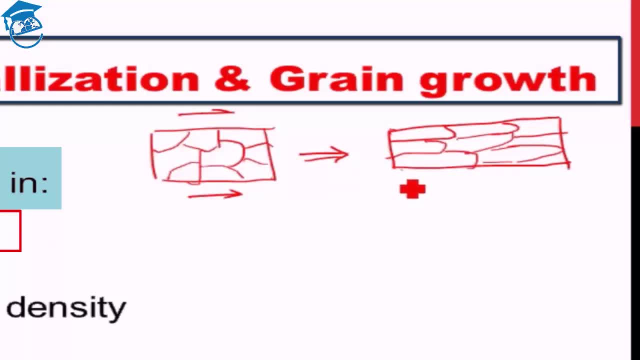 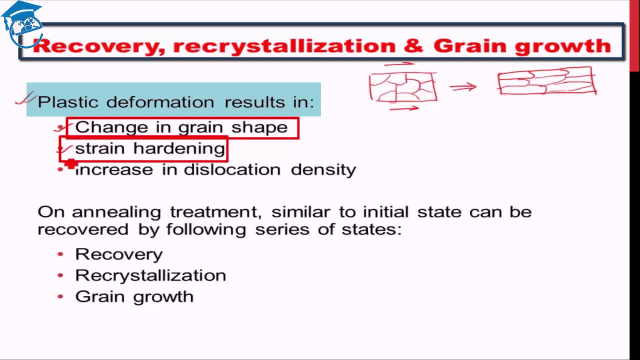 The first thing, This is an observable difference under a microscope. Obviously, as we discussed, it leads to strain hardening due to increase in number of dislocation. and that is the third thing: that there is an increase in dislocation density. Now there is a treatment known as annealing treatment. 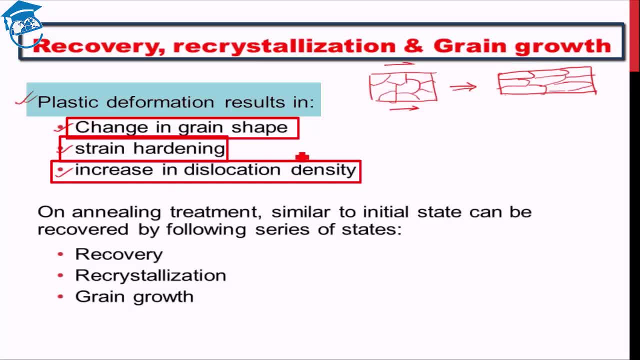 which tries to undo some of the bad effect of plastic deformation In annealing treatment. what we will do. we will see different type of heat treatments later in details. but to give you an idea, in annealing treatment you basically expose the material to a higher temperature and 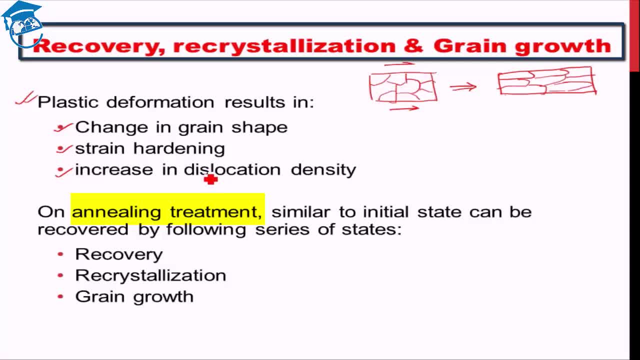 that higher temperature leads to increase in the diffusion processes within the body and that leads to certain phenomena which we will see now. What are the things that can happen? First is recovery will take place in the material. Second is recrystallization will happen. and finally, once recrystallization is done, then 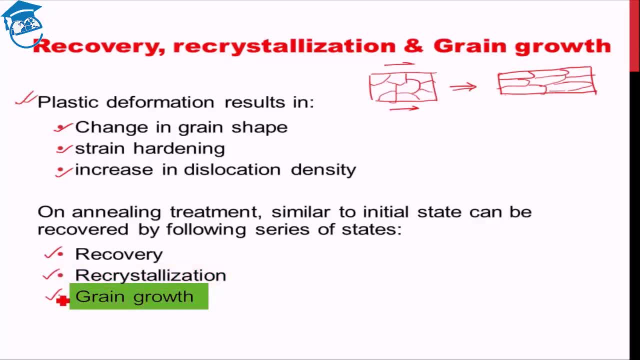 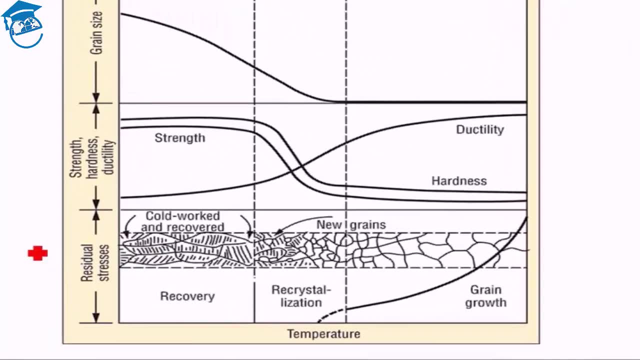 grain growth will take place. Let's see each of them individually. Okay, So this is again. we had a material, we passed it through straightening. We passed it through straightening. So this is again. we had a material, we passed it through straightening. 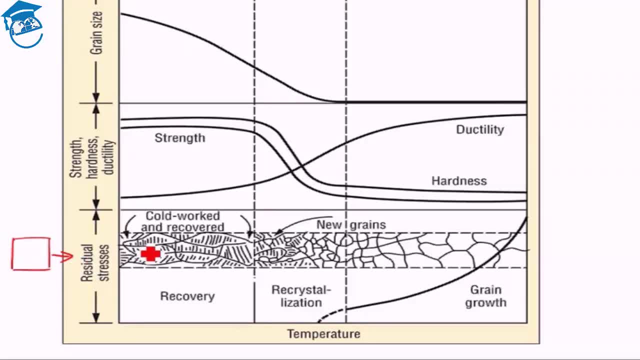 So this is again. we had a material, we passed it through straightening. We passed it through straightening. So this is again. we had a material, we passed it through straightening. So this is again. we had a material, we passed it through straightening. 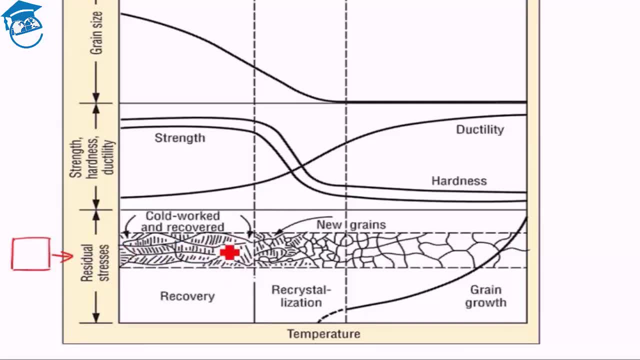 So this is again. we had a material, we passed it through straightening, Okay, And as a result of this cold working, what happened Is that we had with reduced strength and reduction in ductility. Now, the first stage that we have is called the recovery stage. 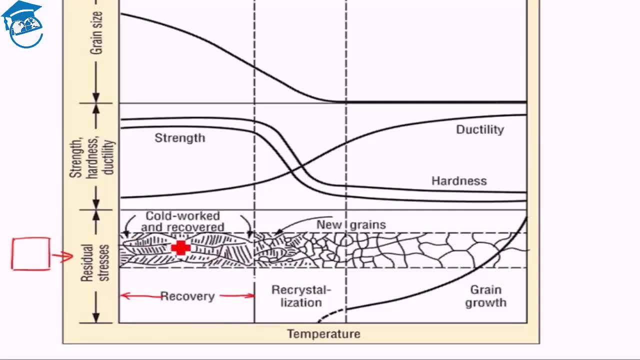 In the recovery stage we will not have any observable difference in the microstructure. The microstructure will manifest. structure will remain elongated as such. But what we will observe is that the ductility is marginally improving. The strength more or less remains the same. 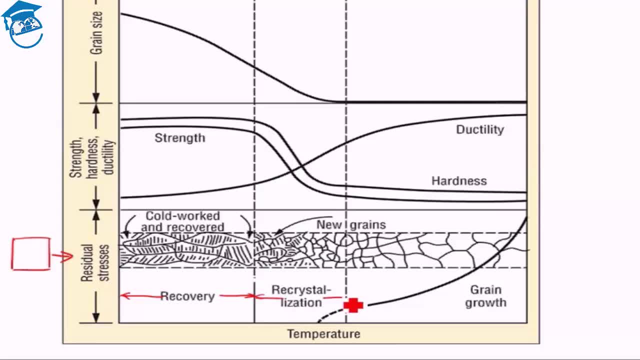 In the second stage, that is, the recrystallization stage, what will be observed is that new grains start to pop up From the old elongated grains. new equiaxed grains start to pop up at different locations And with that the strength of the material starts to reduce, but the ductility 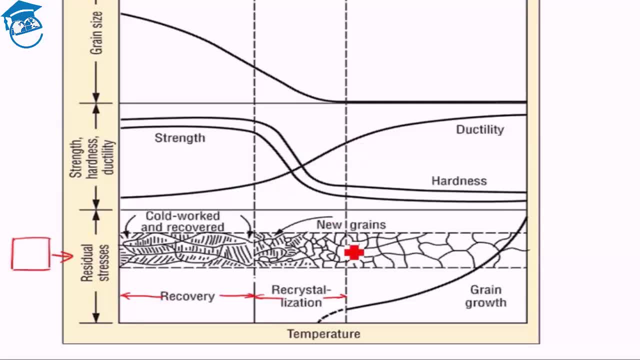 starts to improve drastically. And once we have complete renewal of grains, new grains, then the third stage will happen, where we will have grain growth. Grain growth starts to take place. Smaller grains combine together to form larger grains. Okay, And how is this process taking place? This is basically increase in temperature At lower 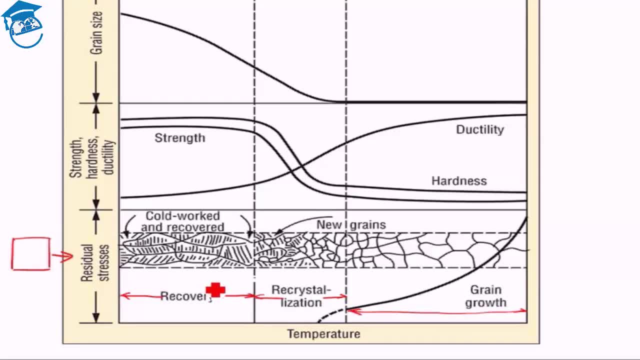 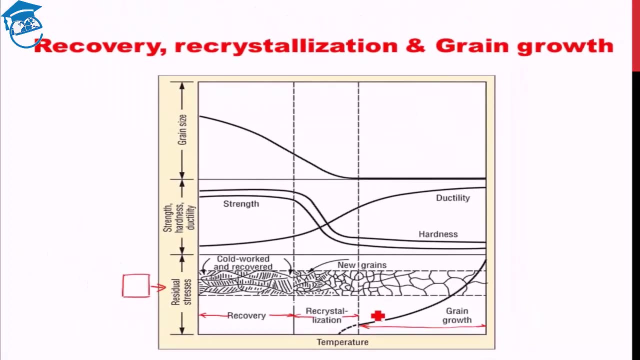 temperature. the recovery stage will be there. Once you reach sufficient temperature, recrystallization will be there, And if you leave it exposed at that temperature for longer time, then grain growth will take place. Fine, Let us see each of them individually now. 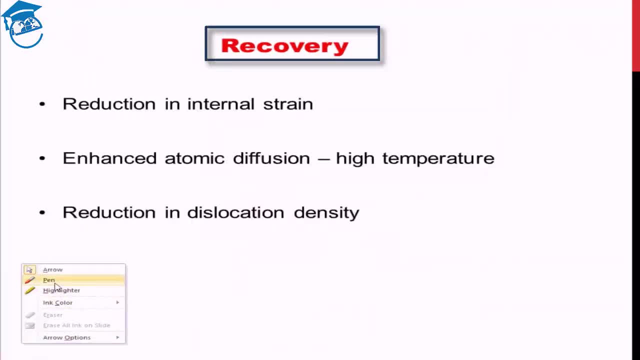 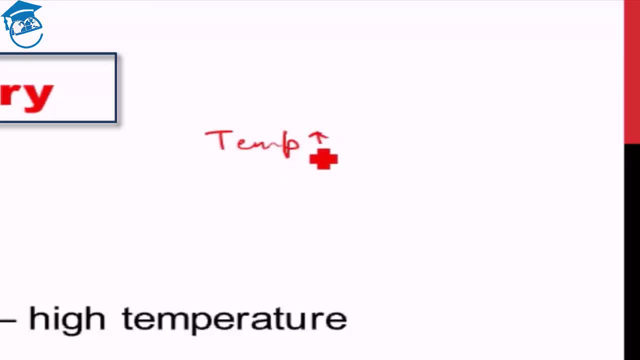 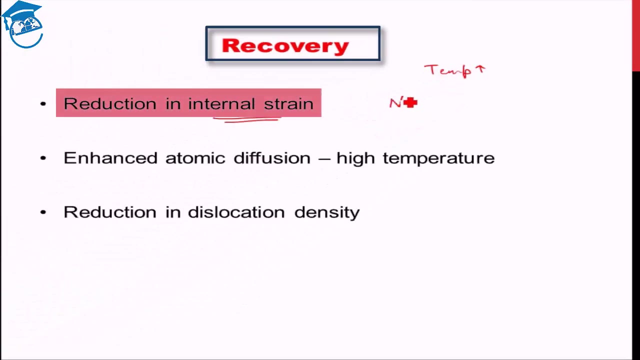 Recovery. In the stage of recovery, what is happening is that you have already exposed it to a little high temperature. Temperature has been increased And this increase in temperature will lead to a reduction in internal strain, But there is no observable microstructural change. No observable microstructural. 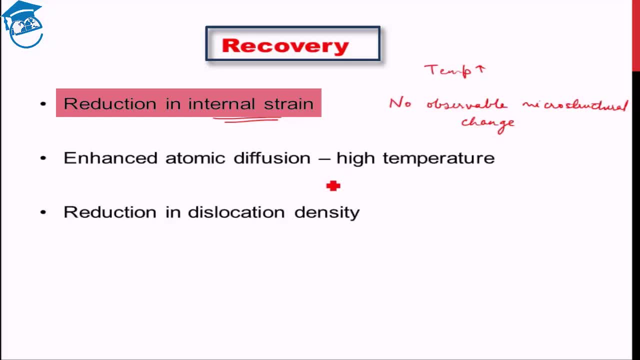 change, but there is a reduction in internal strain. How is that possible? How is the internal strain reduced? The internal strain is reduced or internal stress reduced. That is because at a higher temperature there is enhanced atomic diffusion. Okay, The atoms start to diffuse faster and 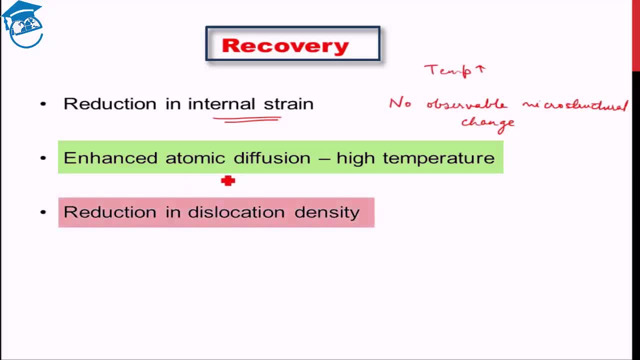 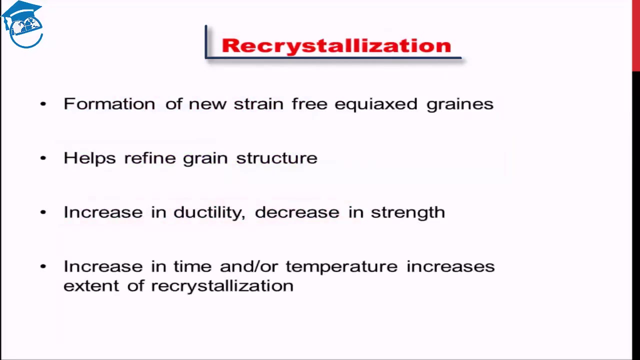 that results in slight reduction in dislocation density and which, as a result, leads to a reduction in internal strain. So this is the idea about recovery. This is the first stage. The next stage which we go is known as recrystallization. 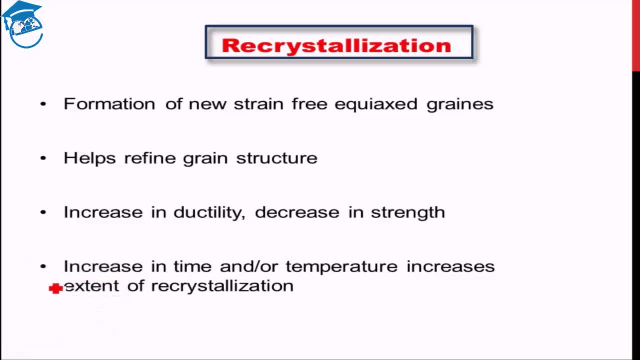 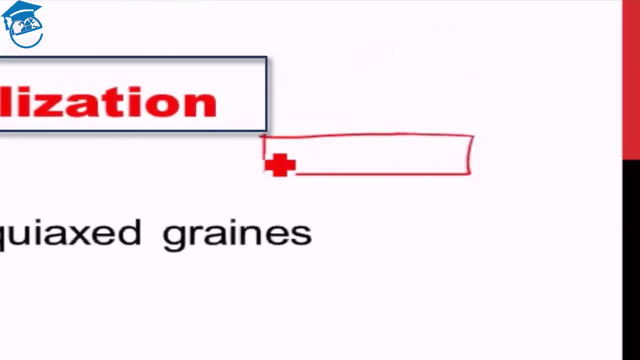 As I have shown in the diagram, a couple of slides back in the stage of recrystallization. what is happening? out of the old grains, from the old grains which were elongated, having a lot of strain within it grains, new grains start to pop up. 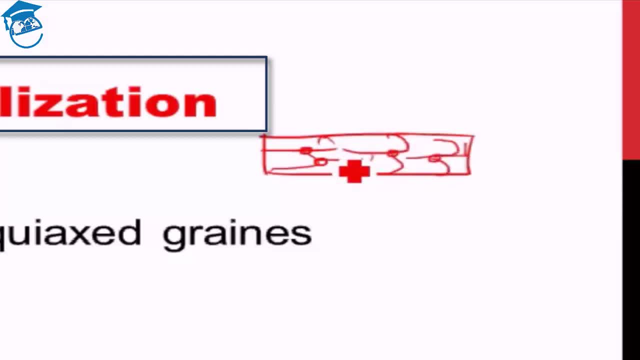 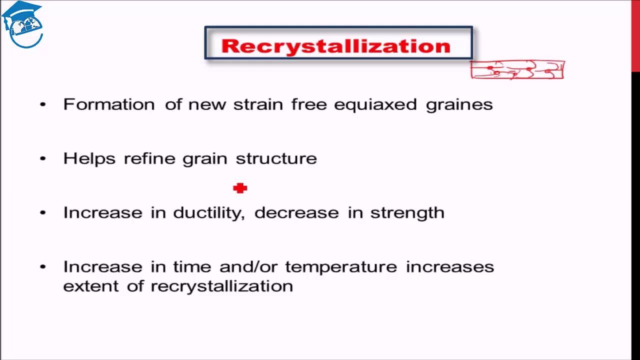 Nucleation of new grains start to take place. Okay, And then this new grains start to pop, start to grow and fresh, refined new grain structure is developed. in this stage Now you will ask: why does new grains nucleate? New grains nucleate because the old grains have a lot of dislocation. 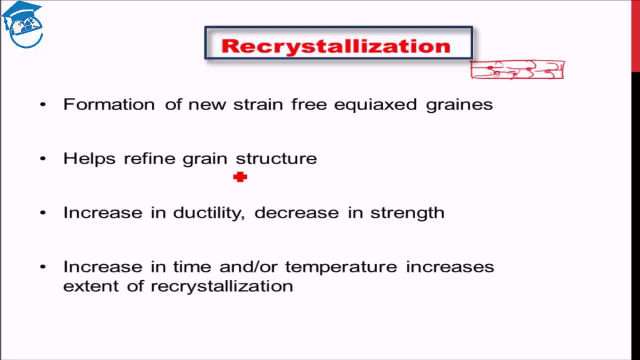 That means it has a lot of energy stored within it. The high temperature at which the material is exposed gives enough activation energy to produce fresh grains which have very low strain within it. thereby it leads to a reduction in the total energy of the system, which is a favorable process. 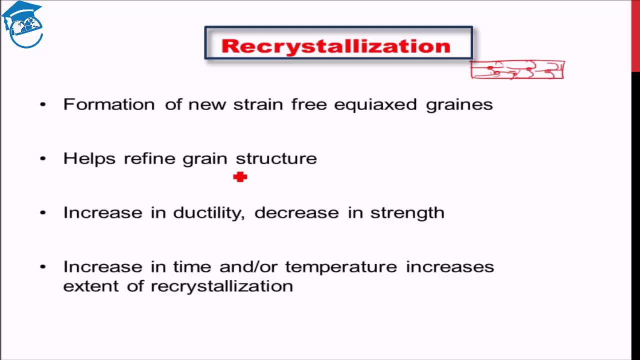 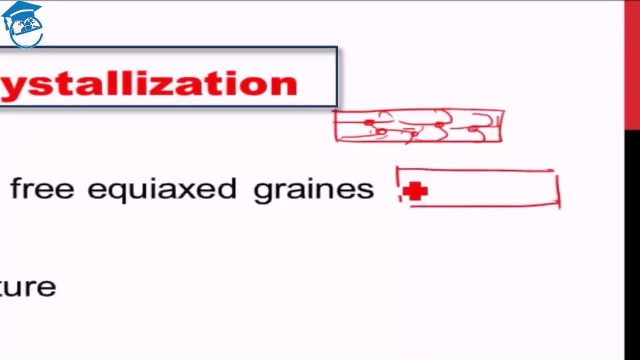 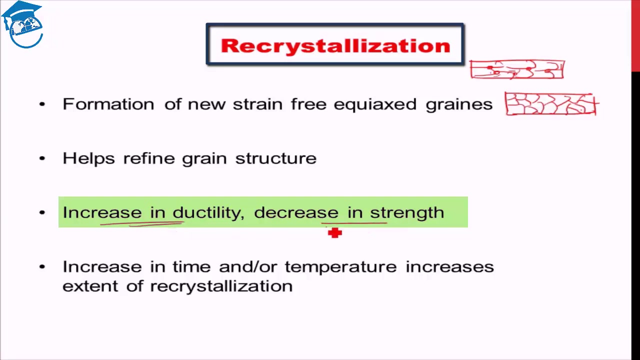 That's why new grains originate And that new grains spread through the material, taking up the whole material and providing very finely distributed, equiaxed new grains. This results in two things: This results in an increase in ductility of the material, but compromises with the strength. 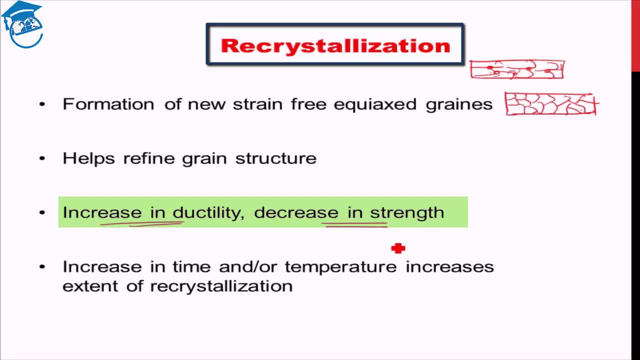 of the material. The strength decreases and the ductility increases, but the decrease in strength is not very high. The increase in ductility is much better and compromises much more than the loss in strength. Why is there a decrease in strength? The decrease in strength is because the dislocation density is reducing. 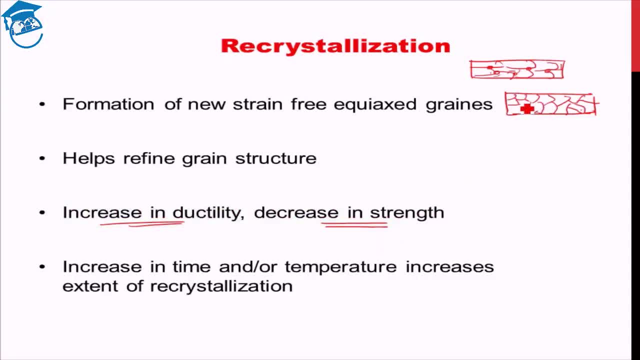 But the idea is that since the grains are very, very fine, then by Hall-Pitch relation, even now the strength of the material will be quite good. The increase in time or the temperature increases the extent of recrystallization. If you expose the material, it increases the extent of recrystallization. 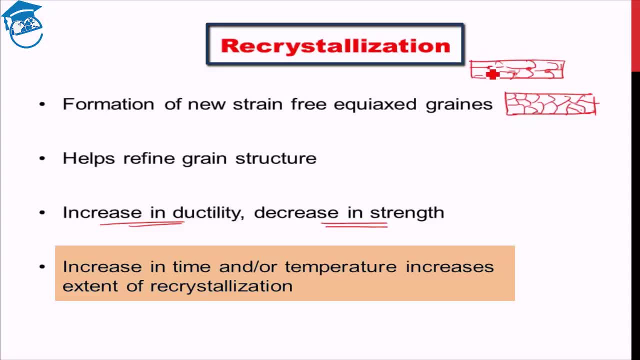 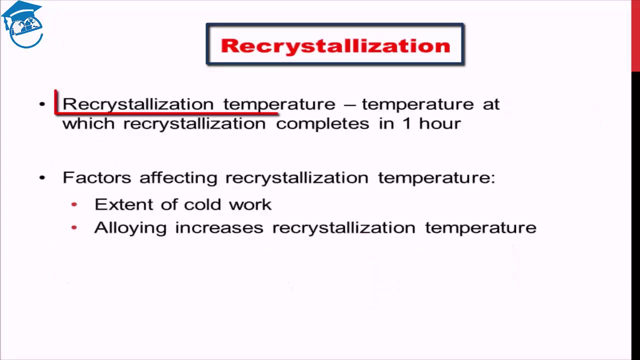 If you expose the material, expose this elongated material, elongated grains, for higher temperature or more time, then the recrystallization can reach towards completion. That is, the whole specimen can become finely renewed, fine grains. Now there is something known as recrystallization temperature. 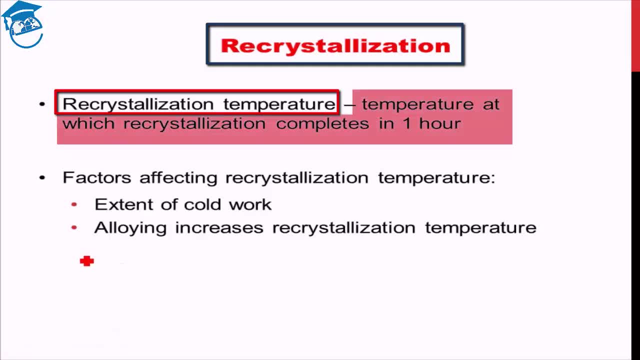 Recrystallization temperature is the temperature at which recrystallization occurs, At which recrystallization can complete in exactly one hour. So what is the temperature where you need to leave the material for one hour for the recrystallization to be complete? 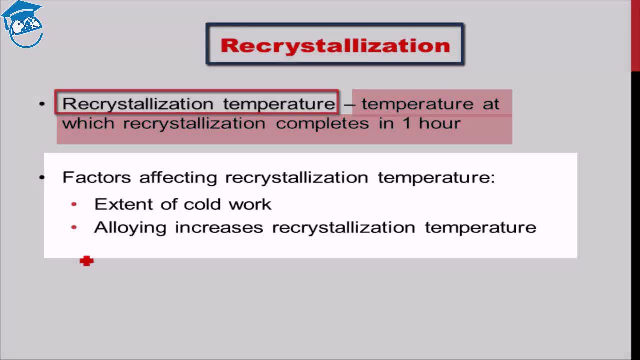 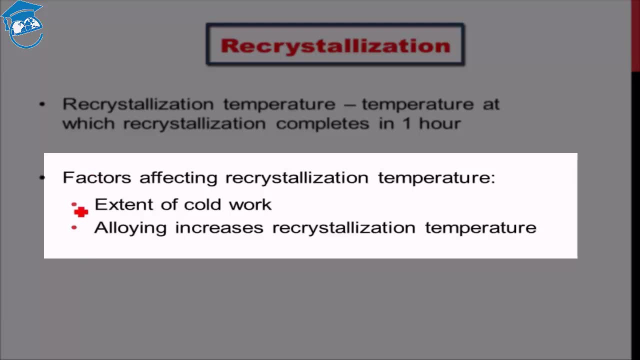 That is known as recrystallization temperature. Now, there are several factors on which recrystallization temperature will depend. The two most important factors are: one, what is the extent of cold work of the material, and second is the temperature. So what is the temperature? 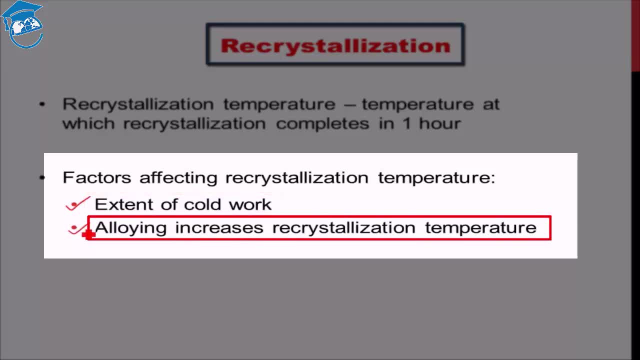 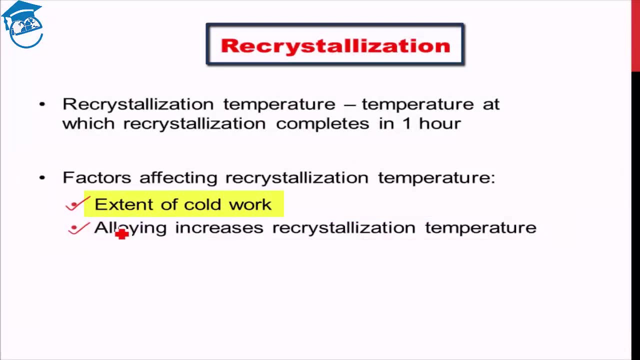 What are the alloying elements or the amount of alloying present in the material? What do we mean by the extent of cold work? See, if you have a material which is 10% cold work and you have another material which is 50% cold work. 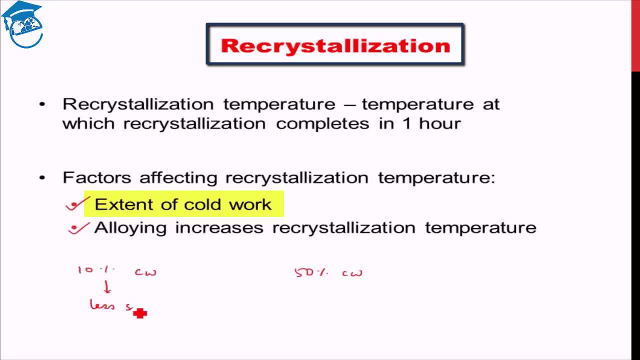 What will happen is this will have less strain. this will have more strain. Therefore the 50% cold work. Since it has more strain, it will have more drive within it, more driving force for the recrystallization to occur. 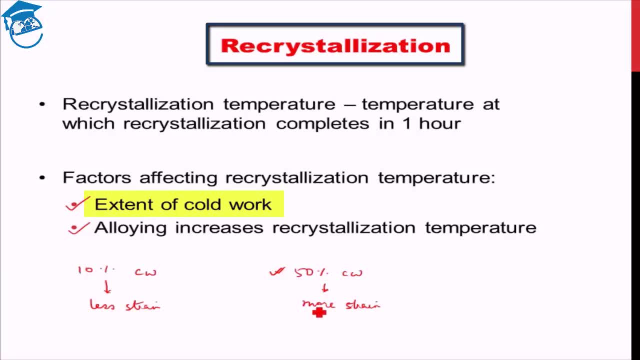 Therefore, more paradoxically, what will happen? a material which has more cold work will actually be easier to recrystallize. More cold work means easier to recrystallize. Therefore, even at lower temperature, more cold work material recrystallizes. 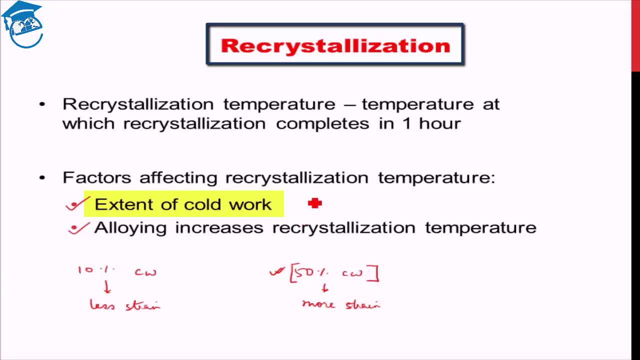 So what is the temperature? What is the temperature? The temperature is not good. The temperature of metal recrystallizes, So high cold work percent, low recrystallization temperature. And the second criteria was alloying. The alloying of a metal leads to an increase in recrystallization temperature. 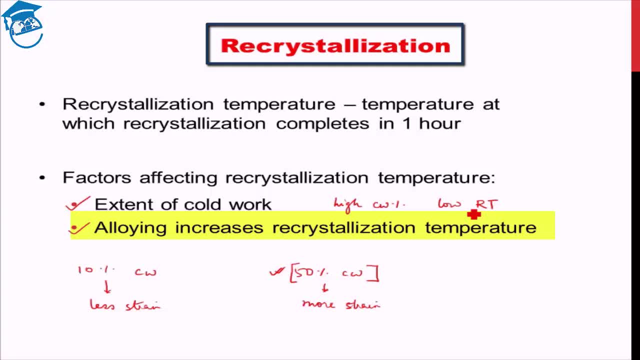 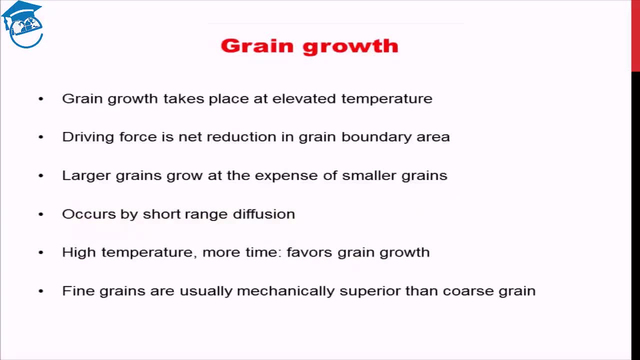 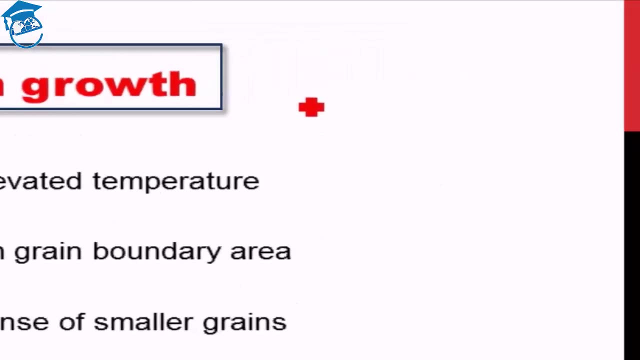 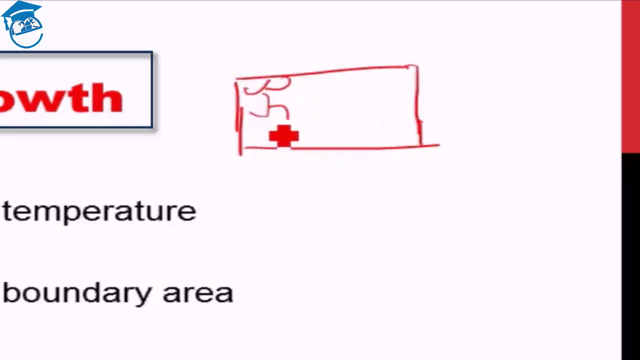 The amount of alloying results in an increase of recrystallization temperature. Fine And final stage is the grain growth. Now that we had recovery and recrystallization, we have fresh grains within the body which are strain free and nicely distributed equiaxed grains. 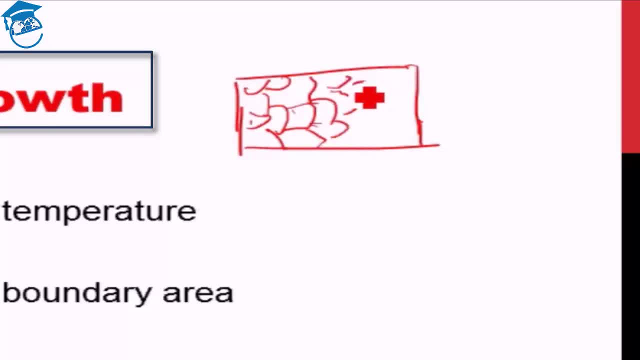 So what now? If we keep the material exposed to high temperature even now, then what will happen is that smaller grains will be consumed by larger grains. The smaller grains will be consumed by larger grains and effectively, the grain size, the average grain size, will increase. 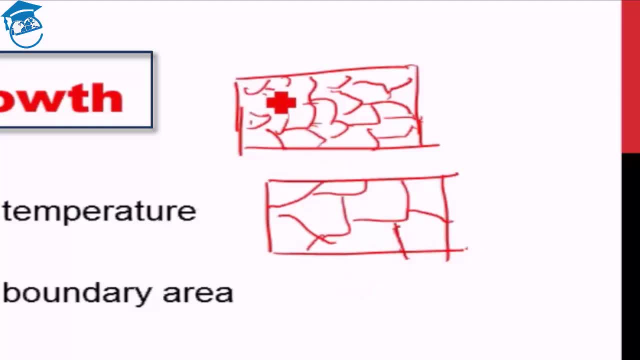 Why is that so? This is so because the grain boundary is region of high energy. Grain boundary is high energy region, So the material wants to get rid of energy. What it will do, It will try to reduce the grain size. Grain boundary area. 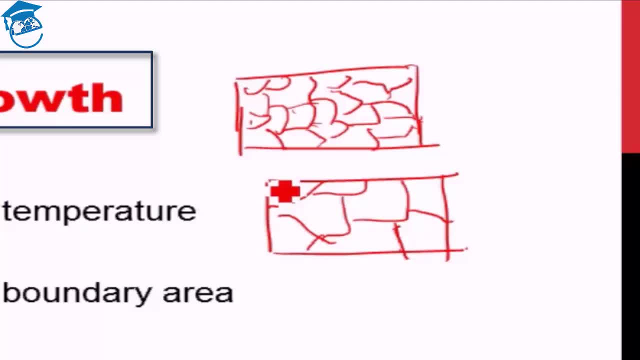 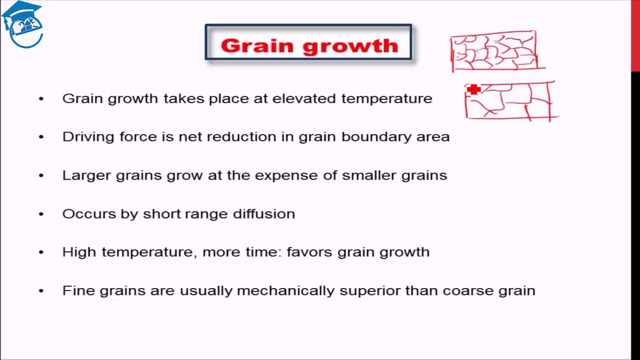 How it can do that. It can do that by consuming smaller grains into larger grains. Larger the average size. less is the effective energy due to the grain boundaries. How does the grain growth happens? Grain growth happens by short range diffusion processes. So what is happening is, if you have a grain here, 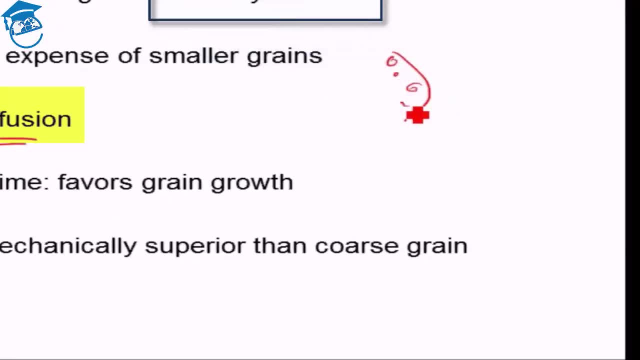 This is the grain. This is the grain With atoms all around here, And another grain here With atoms all around here. So basically, this grain boundary will start to move this way. Atoms move the other way And by this atomic diffusion, basically this grain boundary is moving further out and the 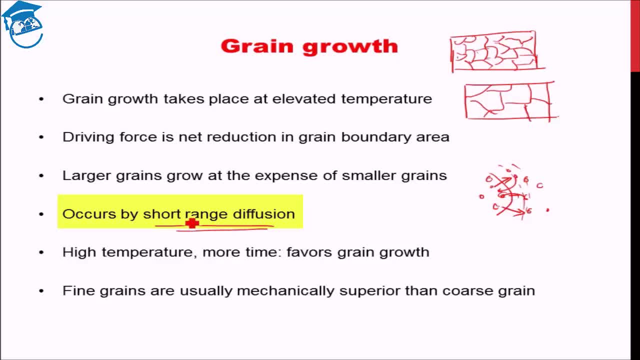 grain size is increasing, So as we see that short range diffusion is involved here, Therefore grain growth occurs at high temperature. It is a kinetic process, So high temperature and more time favors grain growth, But the idea is that grain growth is actually not. 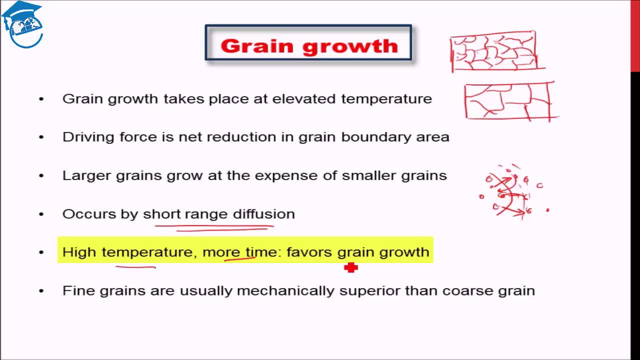 good for the material. By Hall-Petch relation we already know fine grain means more ductile and more strength. Therefore we would rather have fine grain than coarse grain. So we would like to avoid grain growth. Therefore, once we have recrystallization done, we would like 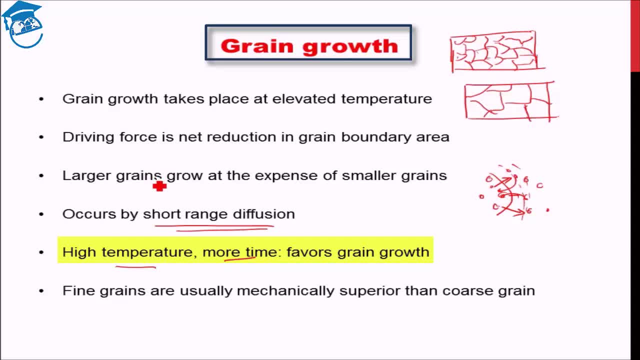 to reduce the temperature so that grain growth does not take place. So this brings us to a conclusion of the discussion. What we have seen today is: we began with the strengthening mechanism, known as strain hardening. We saw that it leads to increase in dislocation.